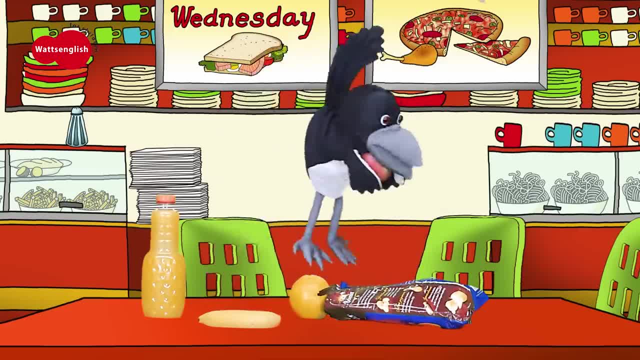 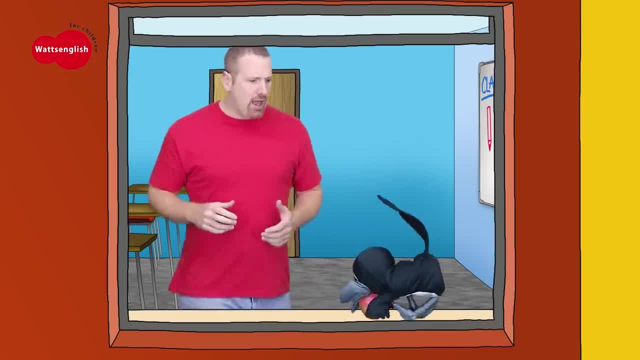 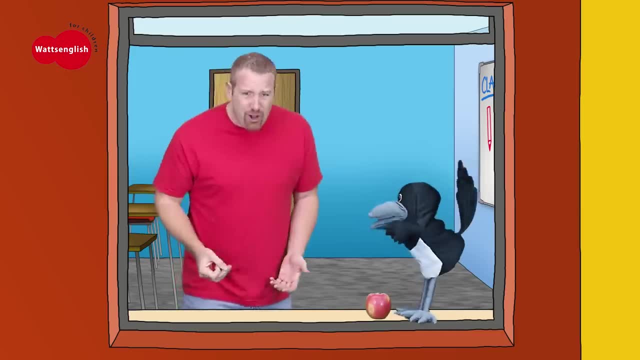 A nice juicy apple. He he, he, Yummy, Yummy. Oh Look, boys and girls, Maggie's coming back. Has she got my crisps? Hey, Maggie, What have you got? A nice healthy apple, An apple, Yeah, An. 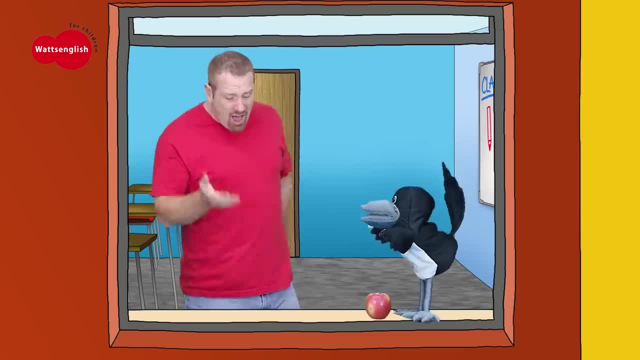 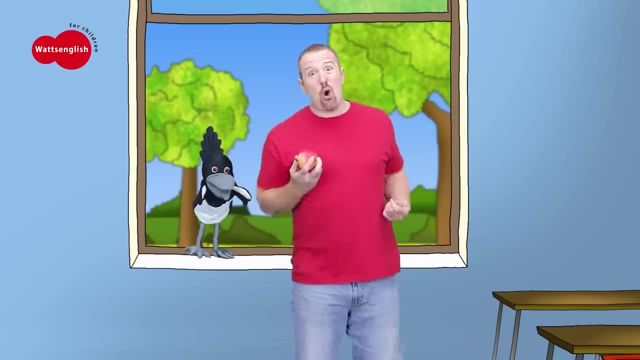 apple? Yeah, Oh, But, Maggie, I don't like apples. Do you like apples? Yeah, Yeah, Oh Well, I'm so hungry, I guess I'll take a bite. Hihi, Mmm, That's delicious Yeah. 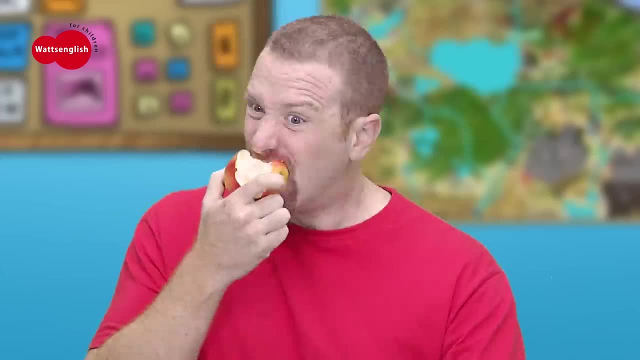 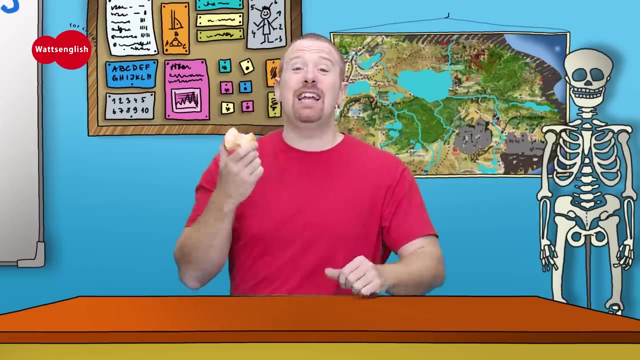 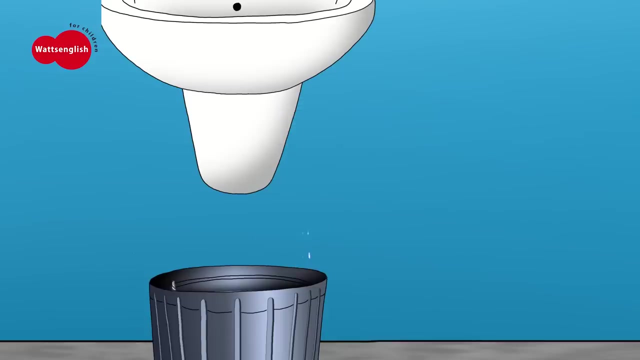 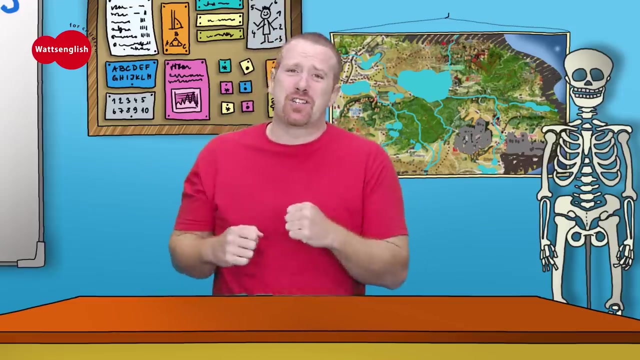 Mmm, Hihihi, Mmm, Mmm. Oh, this apple is delicious. I've forgotten how much I like apples, Mmm, Great, Oh, pardon me, How rude. Oh, that apple was delicious, but I'm still a little hungry and lucky me. 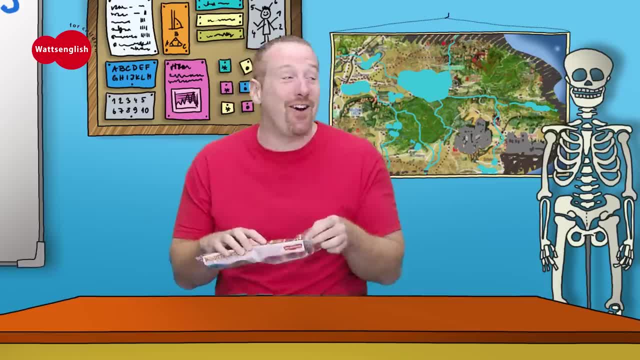 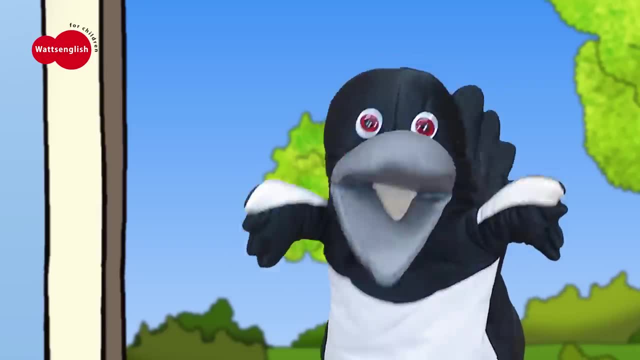 Look down here, I've got some cakes. Oh, Hey, Maggie, Would you like a cake Cake? Oh, I like. cake Cake isn't healthy. Oh, no, no, no, No more cake for Steve Mmm. 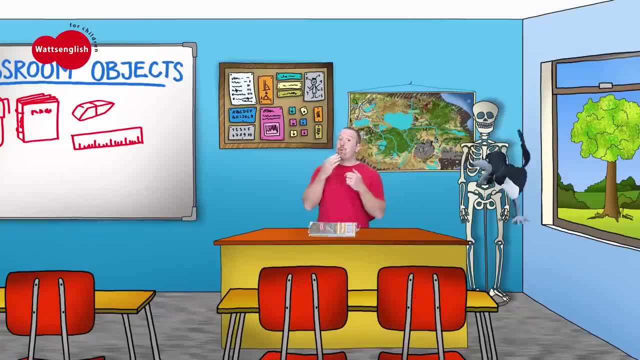 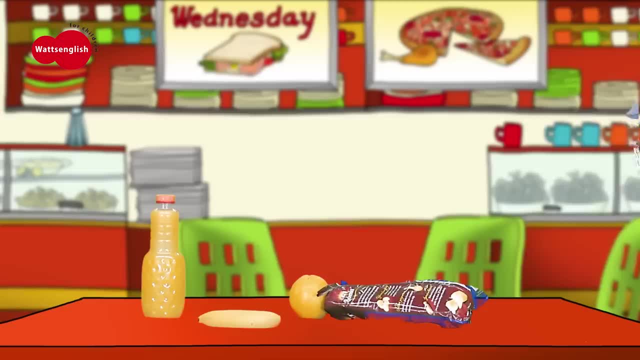 Not my cakes. Oh-oh, I'm saving Steve from a big fat tummy. Oh cakes, So much sugar. Let's give Steve, Oh, a nice juicy orange. Yeah, Hihihi, Oh, Maggie, Oh look. 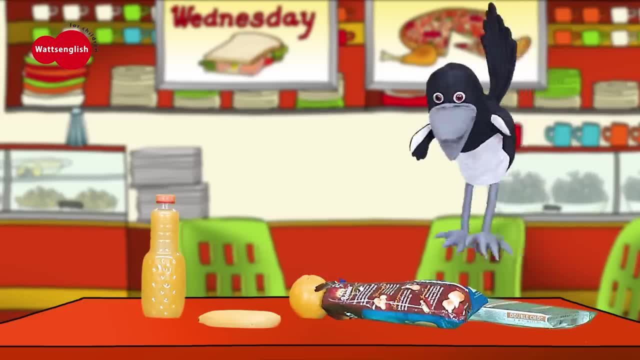 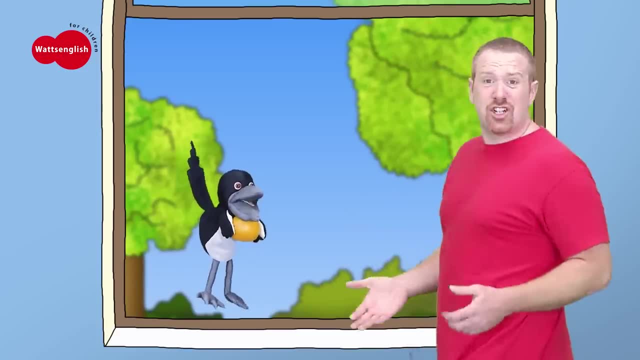 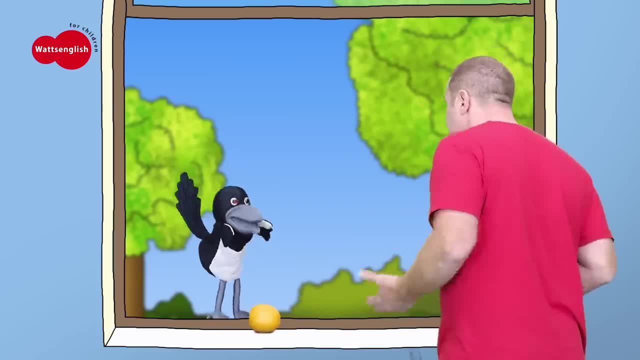 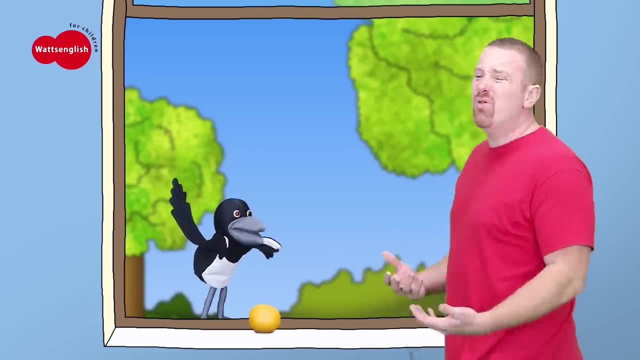 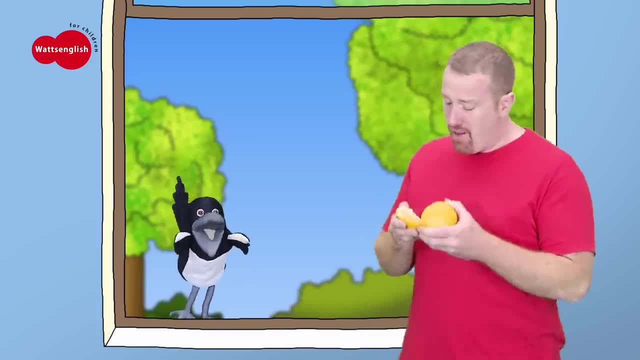 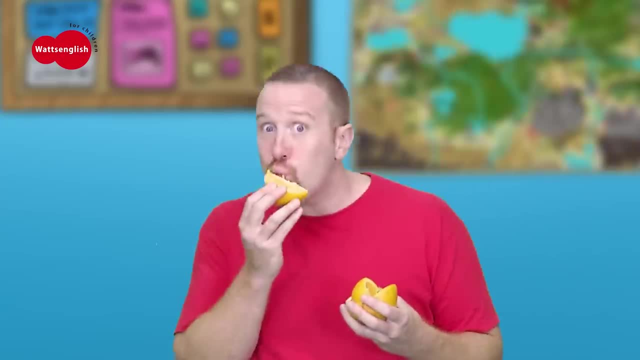 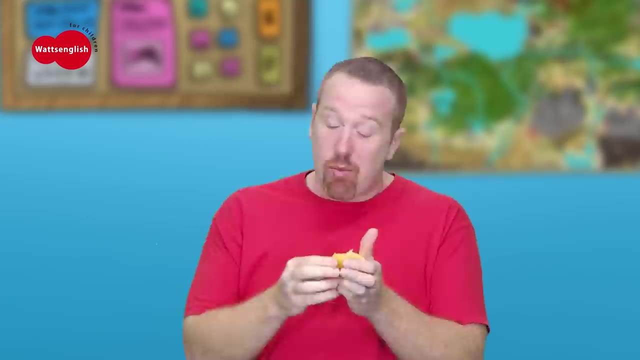 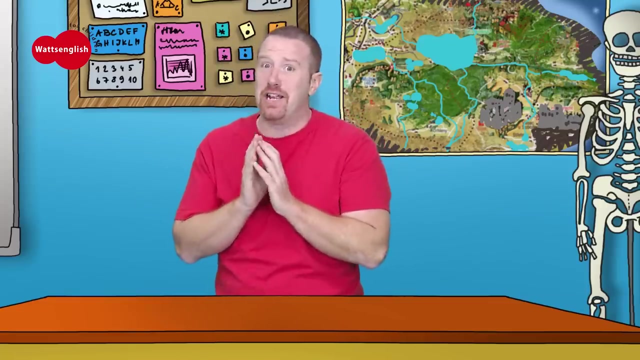 I suppose I should try a little piece of this orange. Yeah, Yum, Yum, Hihihi. Oh, that's great, Mmm, Mmm. Oh, I am very sorry, That was very rude. Well, I had an apple that was healthy and delicious. 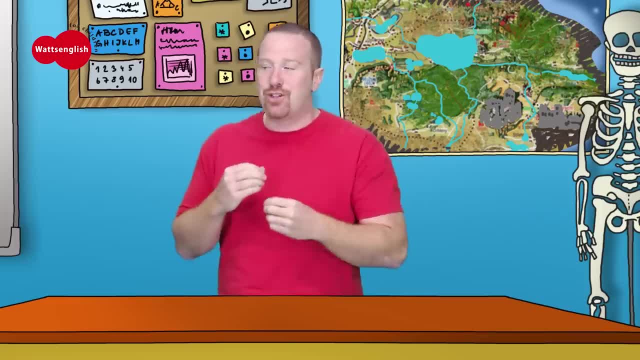 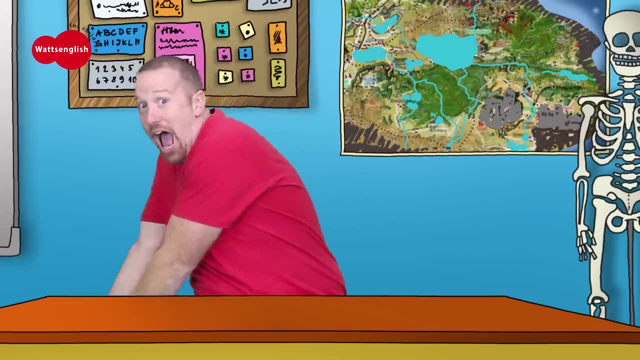 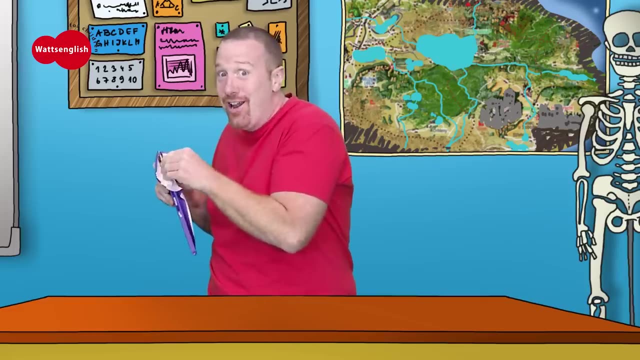 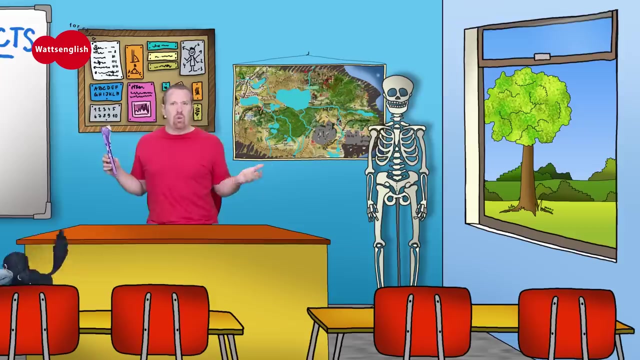 Then I had an orange, which was healthy and juicy, But shhh, don't tell Maggie. I've got one more special treat just down here: Chocolate. Oh, I love chocolate. Do you like chocolate? Hey, Steve, Are you eating chocolate? No, Maggie, It's not chocolate. Hey, where? 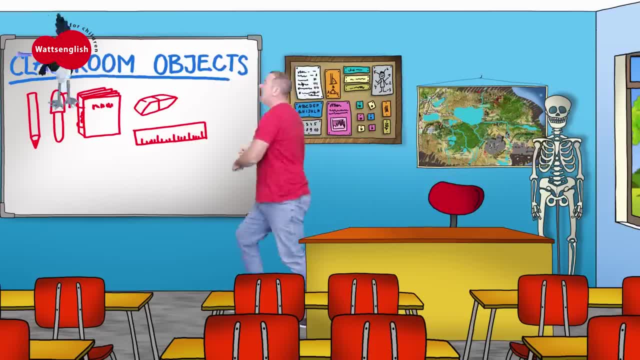 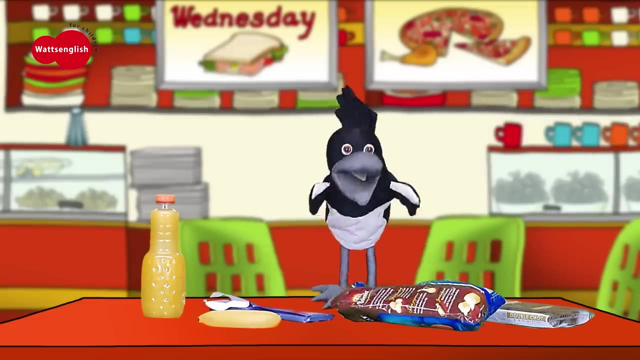 is she? Oh, Maggie, Maggie, give me back my chocolate. No, no more chocolate. No more chocolate for you, Maggie. Oh no, no, I've got to give Steve a healthier snack. Let's give him a banana, Yeah, Great. 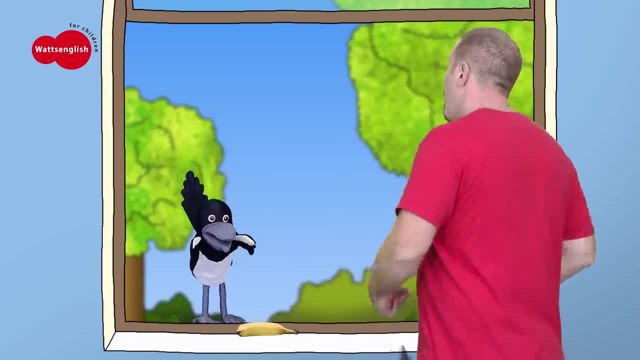 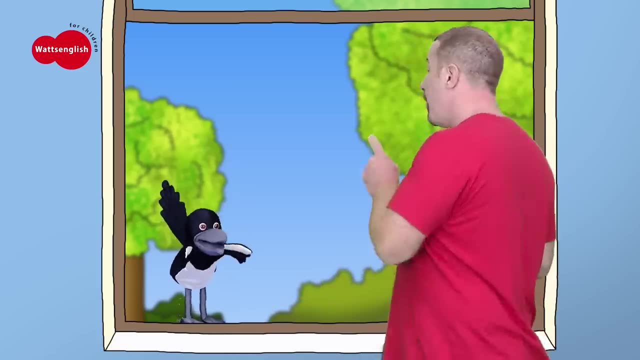 Oh, so, Maggie, you haven't got my chocolate for me. But what have you got? A banana, Yeah, Oh, a banana. Well, I suppose you're right, A banana is a better snack than chocolate. Yeah, I don't want a big, big banana. 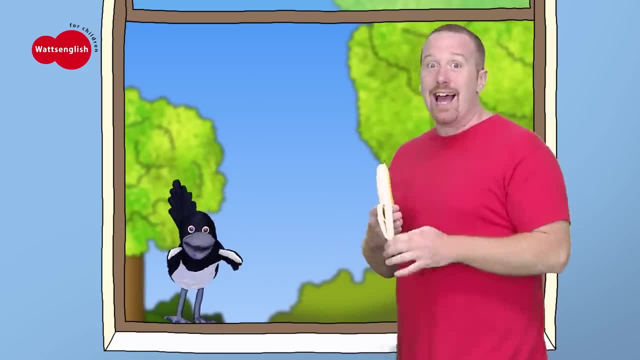 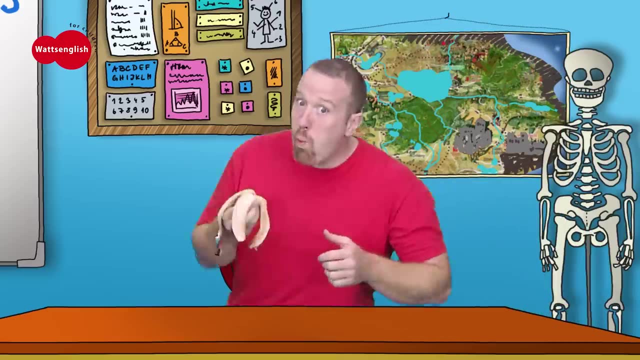 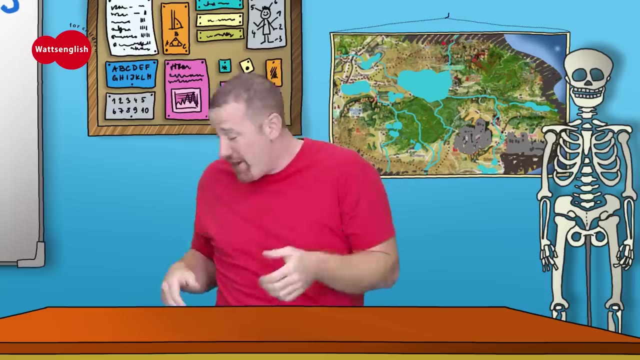 And a fat tummy. No, no, No, no, no. Thanks, Maggie. And anyway, I like bananas. Do you like bananas? Yeah, Mmm, Mmm, Delicious, Great. But now I need a drink And all I've got is… well, this. 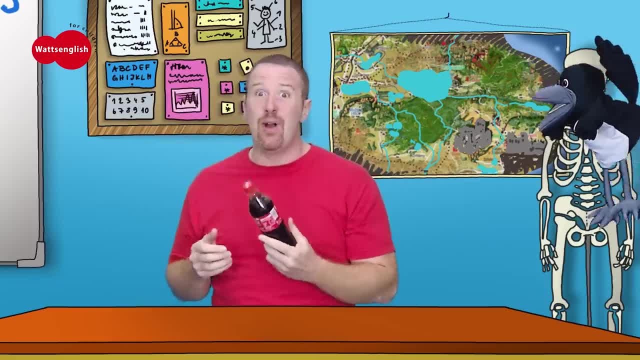 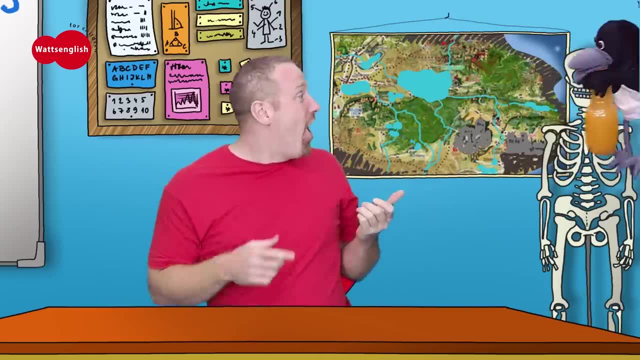 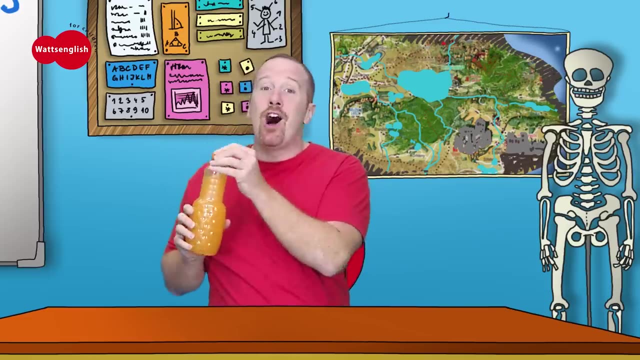 fizzy drink And that's not very healthy. No, It's full of sugar. Oh Hey, I wonder what Maggie will bring me instead. Oh look, Thanks, Maggie. Orange juice, Great Foam- Oh delicious. So now I feel healthy.